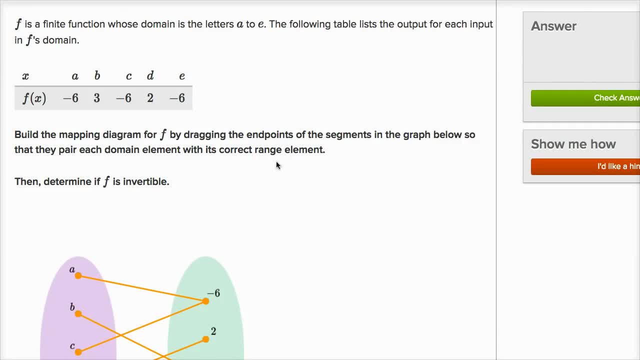 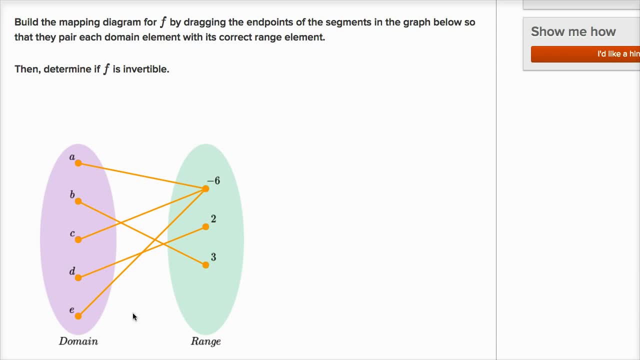 You're going to output two, and then finally, E maps to negative six as well. E maps to negative six as well. So that's a visualization of how this function F maps from A through E to members of the range. but also ask ourselves: is this function invertible? 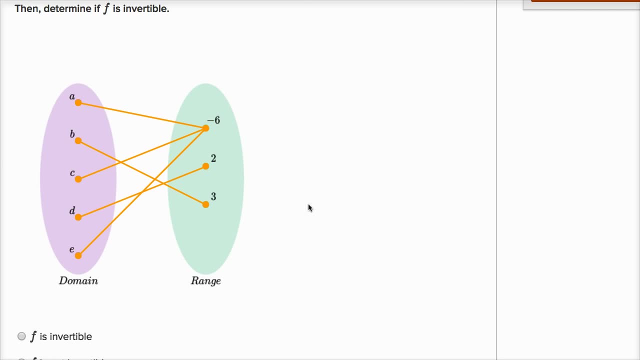 And I already hinted at it a little bit. Well, in order for it to be invertible, you need a function that could go from each of these points to that can do the inverse mapping, But it has to be a function. So if you input three into this inverse function, 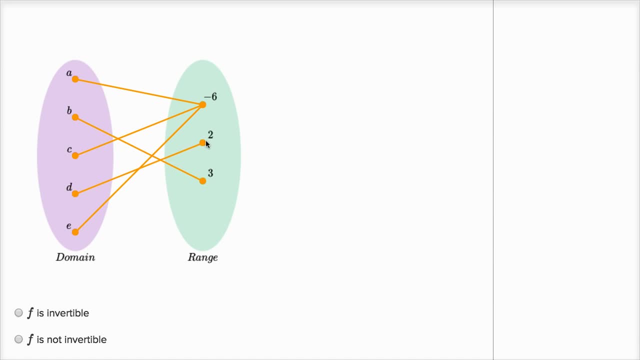 it should give you B. If you input two into this inverse function, it should output D If you input negative six into this inverse function. well, this hypothetical inverse function, what should it do? Well, you can't have a function that, if you input a number, 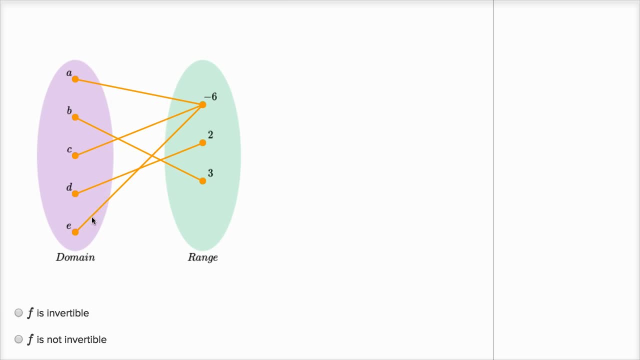 it could have three possible values: A, C or E. You can only map to one value, So there isn't. you actually can't say: let's set up an inverse function that does this, because it wouldn't be a function. 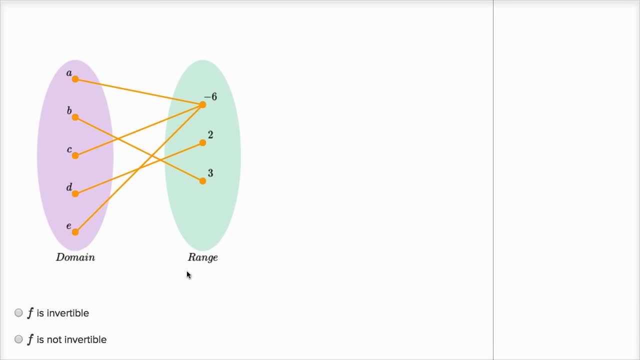 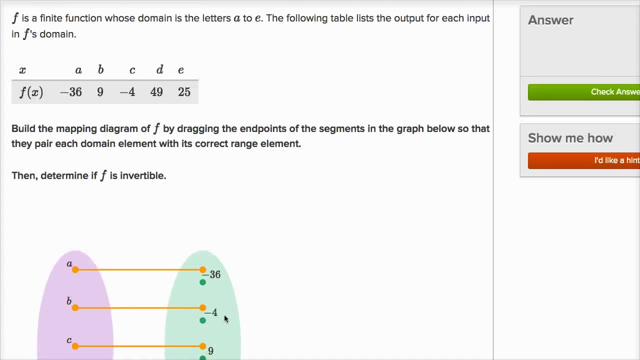 You can't go from input negative six into that inverse function and get three different values. So this is not invertible. Let's do another example So here. so this is the same drill. We have our members of our domain, members of our range. 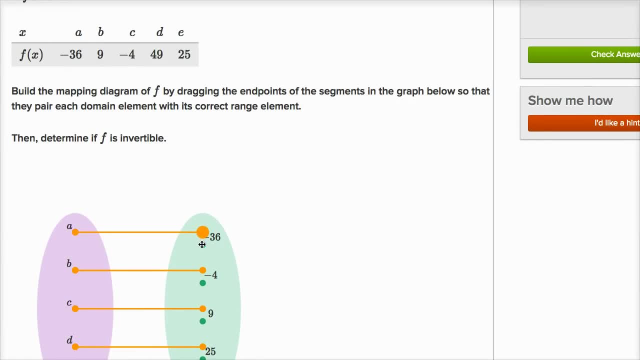 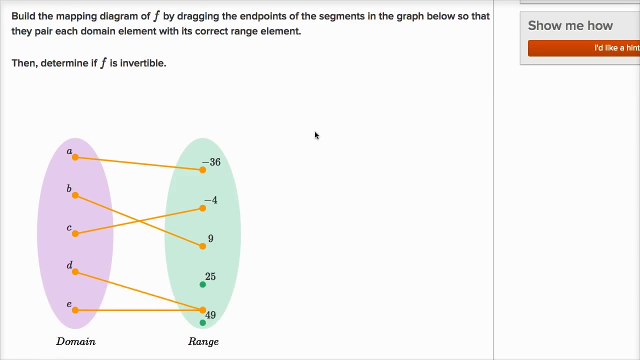 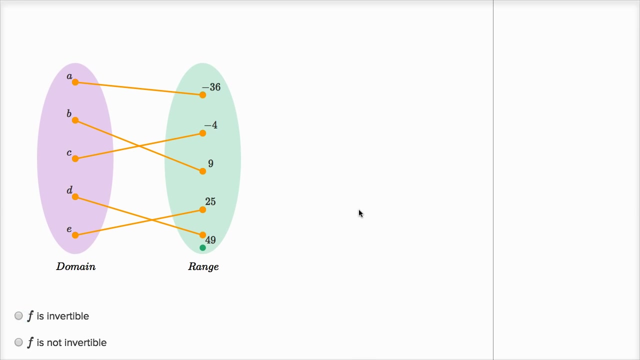 We can build our mapping diagram: A maps to negative, 36.. B maps to nine, C maps to negative four. D maps to 49. And then finally, E maps to 25.. E maps to 25.. Now is this function invertible? 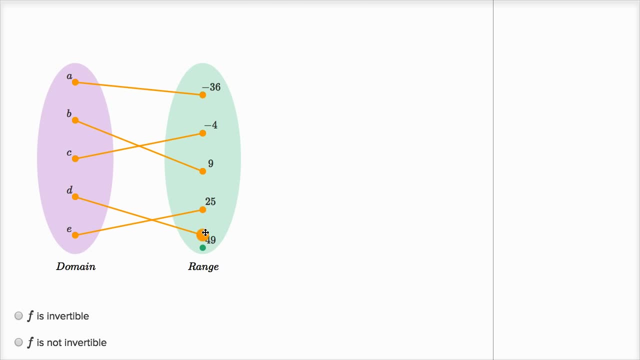 Well, let's think about it. The inverse whoops, the, what was it? D maps to 49.. So let's think about what the inverse, this hypothetical inverse function, would have to do. It would have to take each of these members of the range. 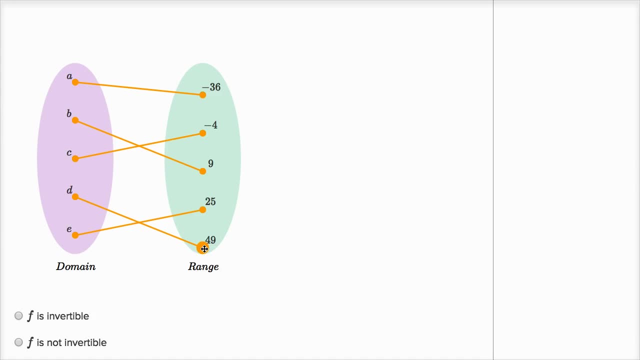 and do the inverse mapping. So if we input 49 into our inverse function, it should give you D, Input 25, it should give you E- Input nine. it gives you B. You input negative four. it inputs C. You input negative 36, it gives you A.